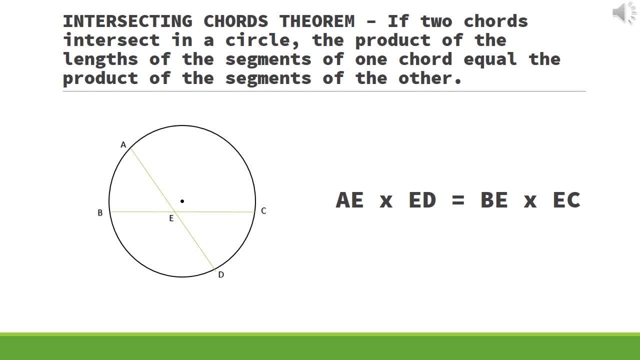 By the intersecting chords theorem. if two chords intersect in a circle, the product of the lengths of the segments of one chord equal the product of the segments of the other. Thus, the measure of line segment AE multiplied by the measure of line segment EB. 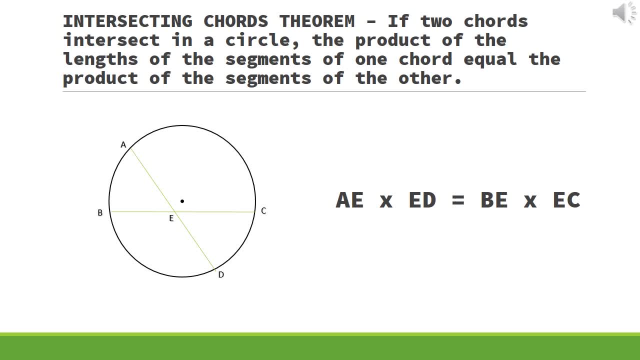 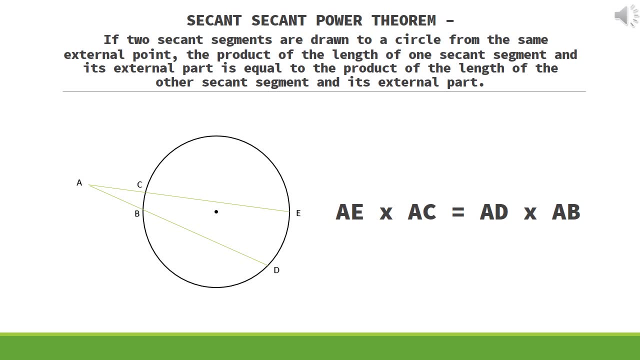 is equal to the measure of line segment BE multiplied by the measure of line segment EC. Now we have a circle with two seconds originating from point A, as shown in the figure By the second-second power theorem, if two second segments are drawn to a circle from the same external point. 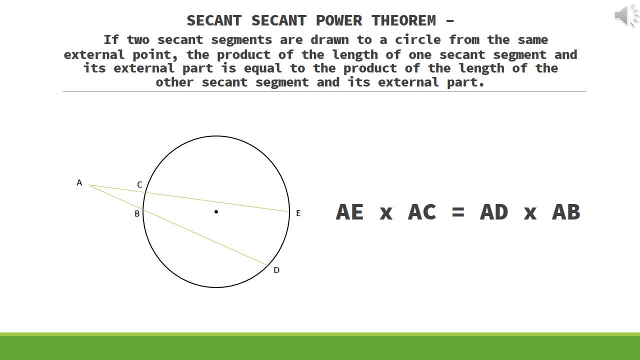 the product of the length of one second segment and its external part is equal to the product of the length of the other second segment and its external part. Thus, the measure of line segment AE multiplied by the measure of line segment AC is equal to the measure of line segment AD multiplied by the measure of line segment AB. 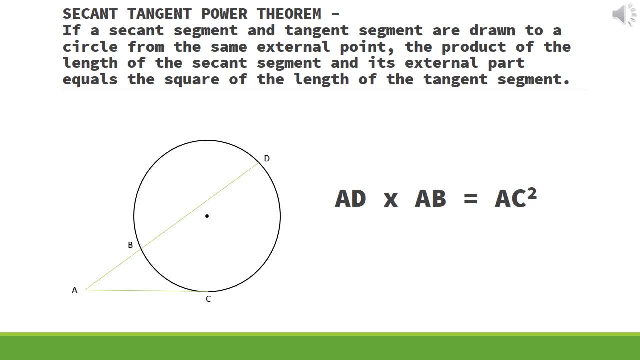 Lastly, consider circle with second AD and tangent AC, as shown in the figure By the second-tangent power theorem. if a second segment and tangent segment are drawn to a circle from the same external point, the product of the length of the second segment and its external part. 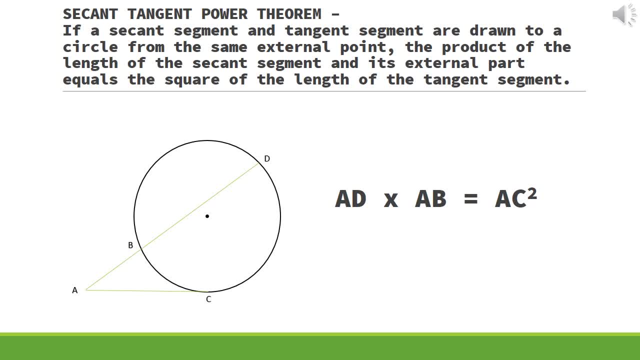 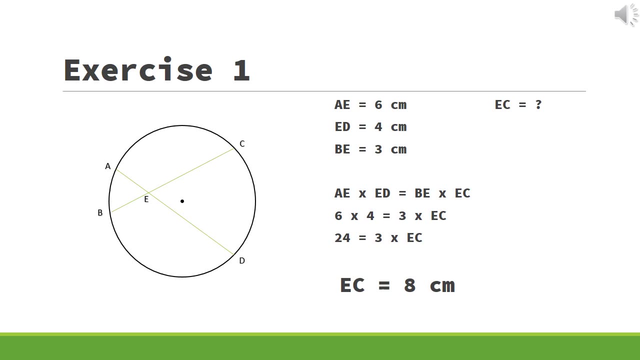 equals the square of the length of the tangent segment. Thus, the measure of line segment AD multiplied by the measure of line segment AB is equal to the square of the measure of line segment AC. Consider the circle with two chords, AD and BC, as shown. 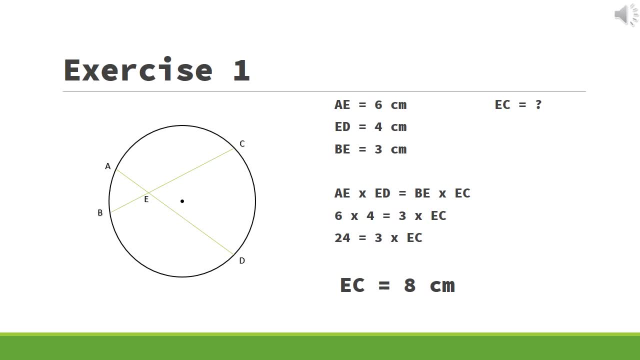 If AE measures 6 cm, ED measures 4 cm and BE measures 3 cm, what is the measure of EC Using the intersecting chords theorem AE times ED is equal to BE times EC Substituting values. 4 times 6 is equal to. 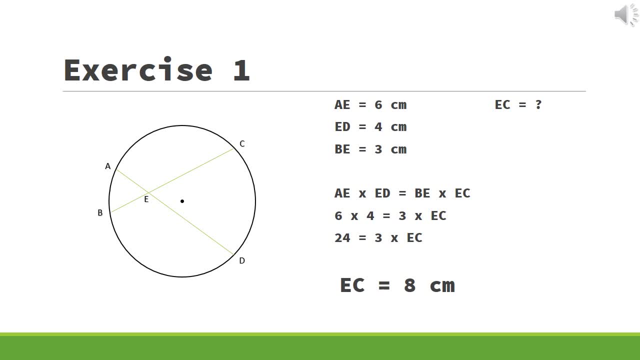 3 times the measure of BC and 3 times the measure of AC. 4 times 6 is equal to 3 times the measure of BC and 4 times the measure of EC. EC, So 24 is equal to 3 times the measure of EC. Dividing both sides by 3, we get that.